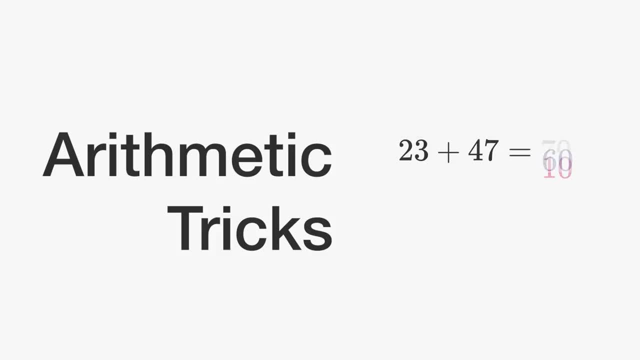 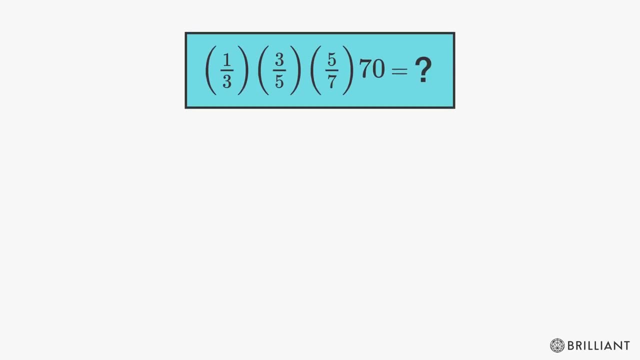 Do you know the quick way to solve this equation? You could just start calculating from the left, but this requires multiplying and simplifying a lot of fractions. Ultimately, it takes a lot of work. The faster way is to take a second to strategize What might have taken a minute or 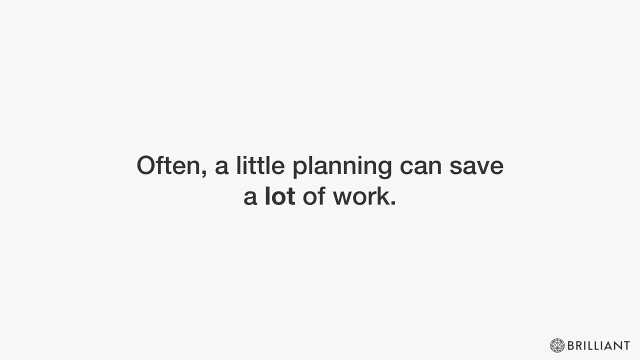 two. the first way takes just seconds. this way, A little planning can save a lot of work. Now try to find the shortcut here. You can split these two numbers into a few smaller ones that are easier to calculate. Now try to find this shortcut on your own. Here's a hint. Find more tricks to save time at Brilliantorg.